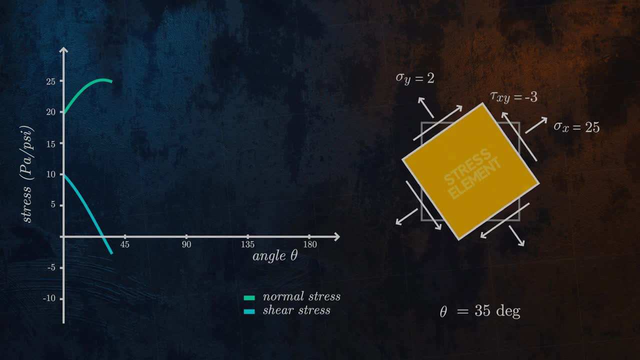 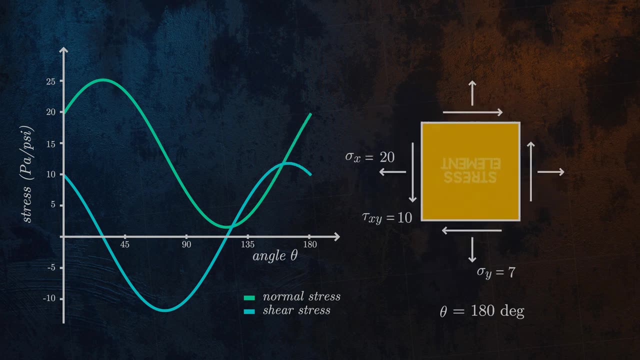 As we rotate the stress element, the normal and shear stress components will vary. Once we have rotated the stress element by 180 degrees, we will return to the configuration we started with. It is important to remember that the actual stress state within the large body is not changing when we rotate our stress element. 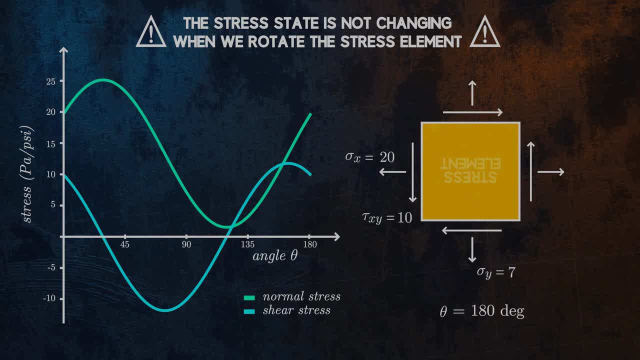 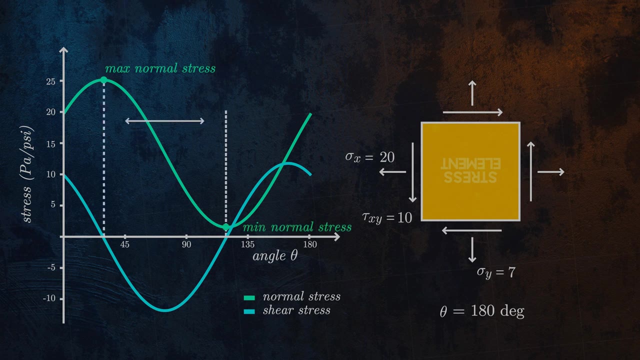 We are just rotating the axes of the coordinate system we are using to visualize the stresses at a single location. We can observe that for certain angles, the normal stress will reach maximum and minimum values, and that these maximum and minimum values are separated by an angle of 90 degrees. 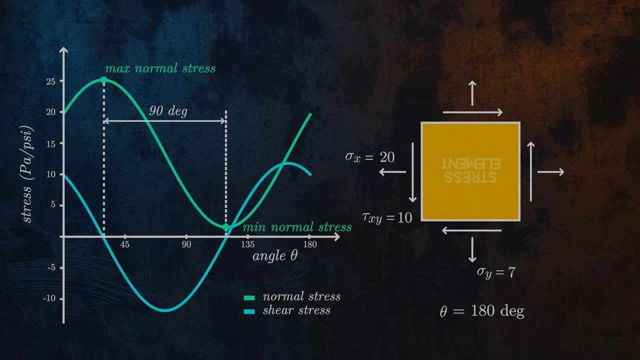 This means that when we rotate our stress element such that we have the maximum and minimum values, and we have the maximum normal stress on the X face of our element, we always have the minimum normal stress on the Y face. Another interesting observation is that when the normal stresses are at their maximum or minimum values, 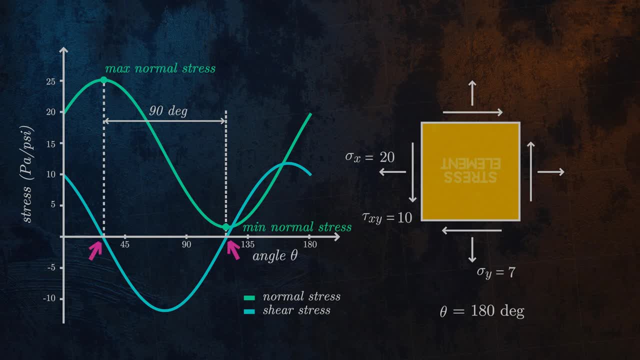 the shear stresses are zero. These faces on which the shear stresses are zero are called the principal planes, and the corresponding maximum or minimum normal stresses acting on these planes are known as the principal stresses. Principal stresses are very important, so let's recap. 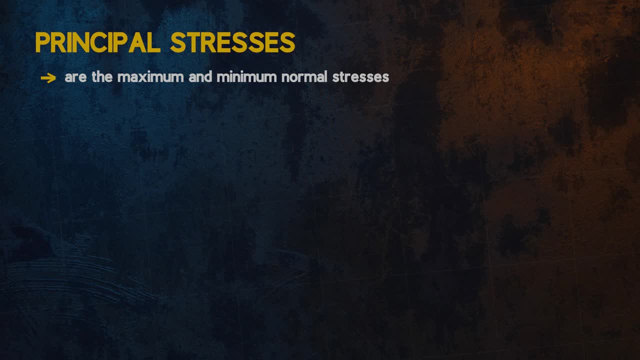 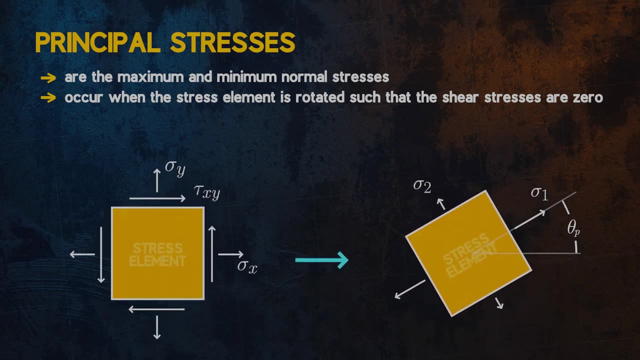 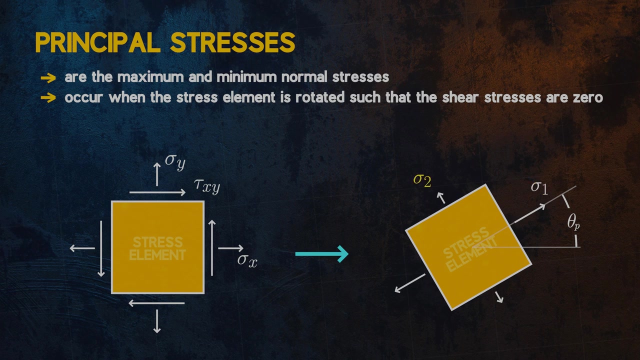 They are the maximum and minimum normal stresses acting on our stress element. They always occur when the stress element is rotated, such that the shear stresses are zero. as shown here, We denote the maximum and minimum principal stresses using the symbols sigma 1 and sigma 2 respectively. 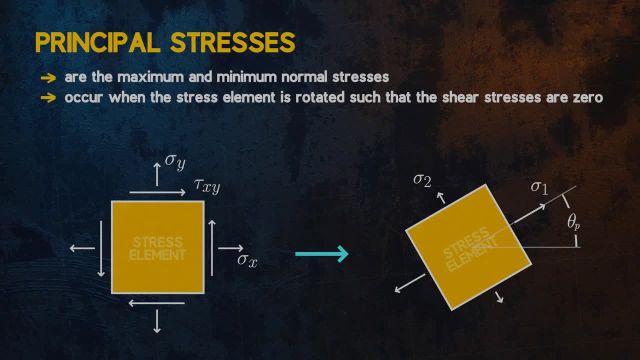 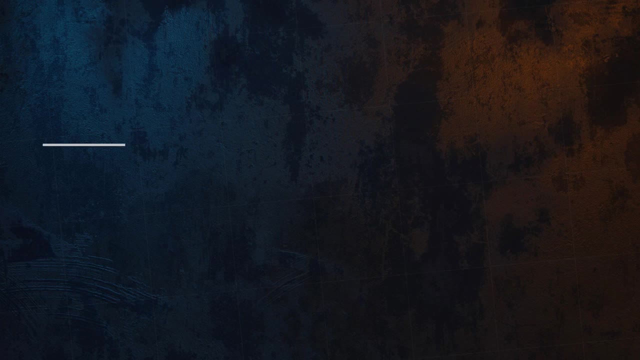 The rotation angle which gives us the principal stresses is denoted using the symbol theta p, Because it is the maximum normal stress at the location of our stress element. being able to calculate sigma 1 can be important for predicting failure. Moore's circle is a graphical method for easily determining the normal and shear stresses. 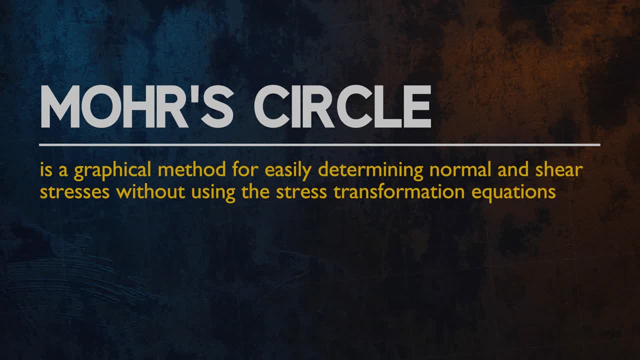 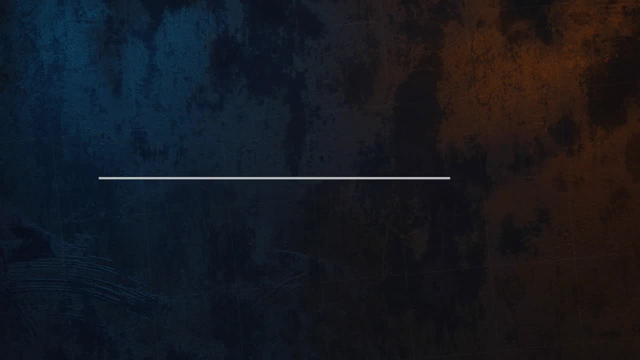 for different orientations of our stress element without having to use the stress transformation equations. Let's see how Moore's circle is constructed. First, let's draw the horizontal and vertical axes. Normal stress is on the horizontal axis and shear stress is on the vertical axis. 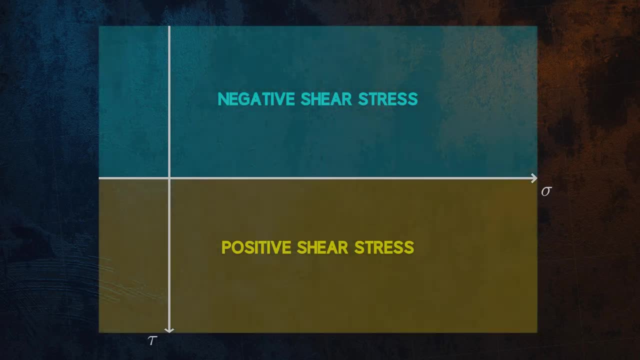 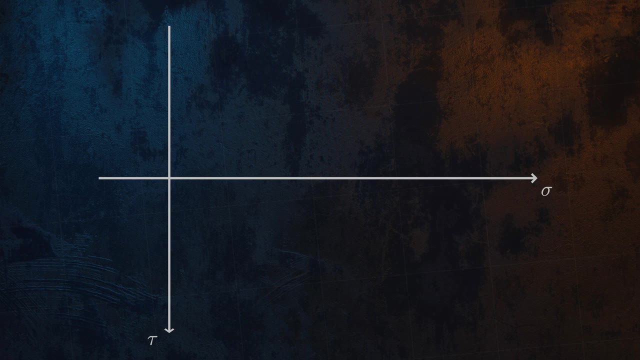 We will plot positive shear stresses in the downwards direction. Next we plot the stress conditions corresponding to the x-face of our stress element by plotting a point with coordinates sigma x, tau, xy. Then we plot a point corresponding to the stress conditions on the y-face. 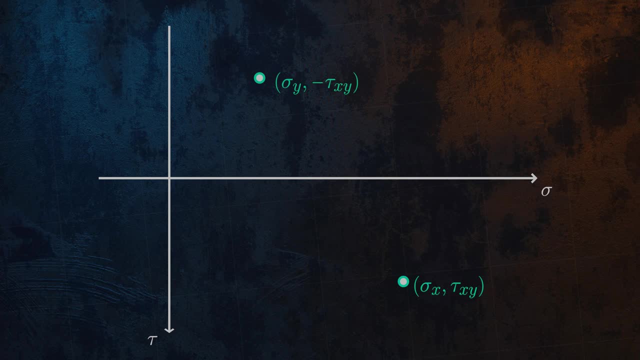 by plotting a point with coordinates: sigma y, negative, tau xy. The sign convention we use for Moore's circle is that shear stresses are positive if they tend to rotate the stress element counterclockwise and are negative if they tend to rotate it clockwise. 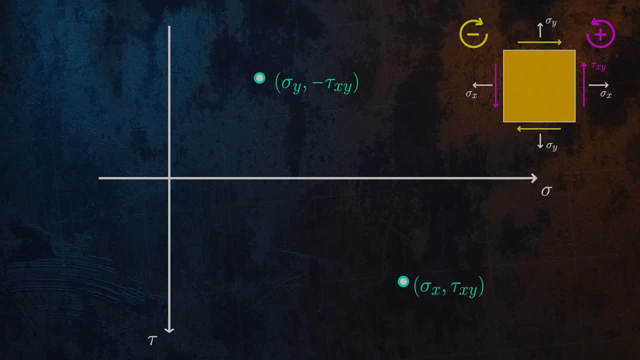 This is why tau xy is negative on the y-face of our element. when we draw Moore's circle, Normal stresses are positive if they are tensile and negative if they are compressive. The line between these two points defines the diameter of our Moore's circle. 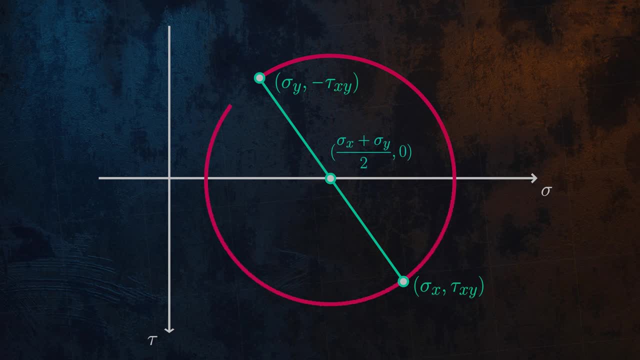 which we can now draw. Each point on the circle represents the normal and shear stresses of our stress element. We can use Moore's circle to work out some interesting information. We can see visually that the maximum shear stress is equal to the radius of the circle. 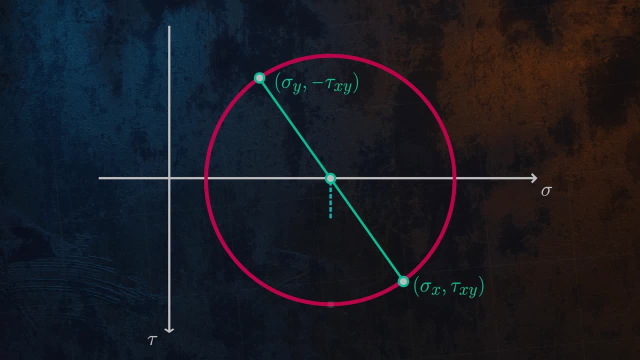 which we can easily determine either approximately by measuring the distance on paper or exactly by using the equation for the radius of a circle. We can also determine the principal stresses by looking at where the circle crosses the horizontal axis, as the shear stress is zero at these locations. 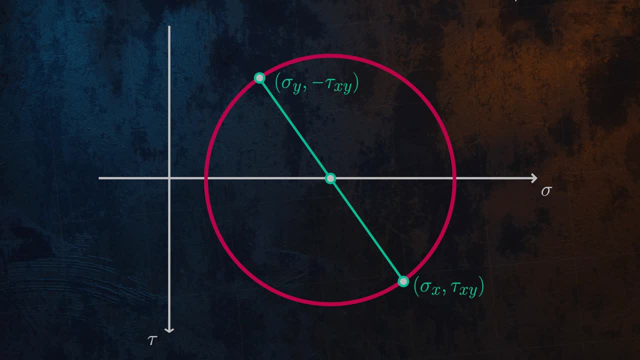 We can also determine the principal stresses by looking at where the circle crosses the horizontal axis, as the shear stress is zero at these locations. The principal stresses can be calculated by taking the x-coordinate of the center of the circle and adding or subtracting the circle radius. 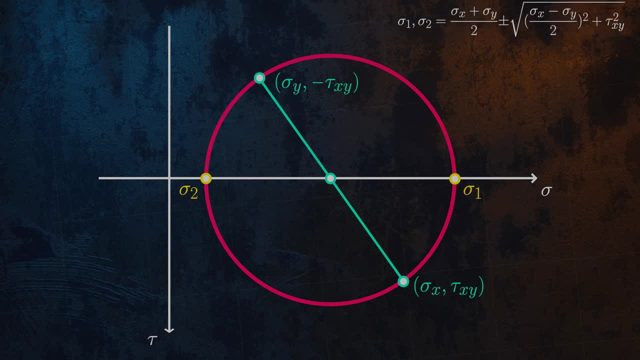 We can also use trigonometry to calculate angles on Moore's circle. For example, we can calculate the angle, theta p, between our original stress element and the principal planes. An important thing to note is that angles in Moore's circle are doubled compared to the angle we rotate our stress element by. 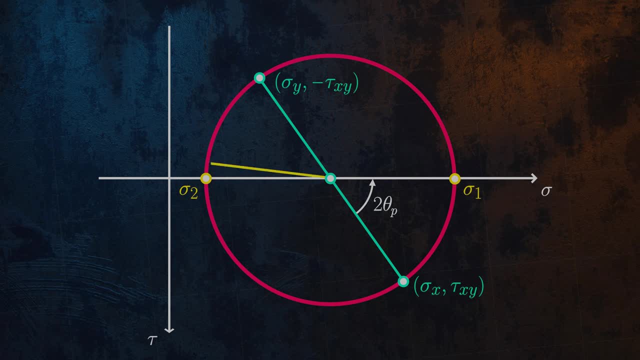 This is apparent by observing that in Moore's circle there is a 180 degree angle between the minimum and maximum principal stresses, whereas on our stress element the angle is 90 degrees. This is why we use the 2 times theta notation on Moore's circle.